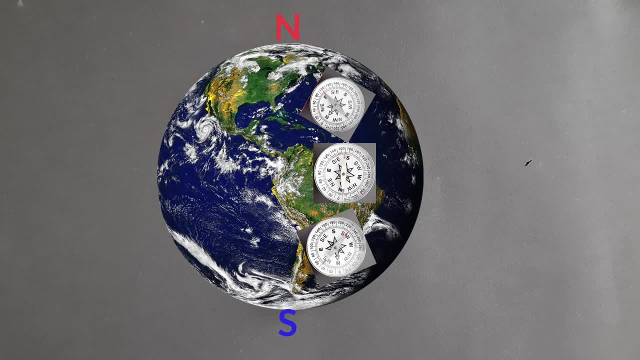 earth today in our world. So many other other connections, like gegen Turkey to the North pole of the earth. even in known that earth acted as a magnet, though the Arcturus bronze like to be a magnetic compass, but i was not方isation of why the earth익ed beятn on earth. 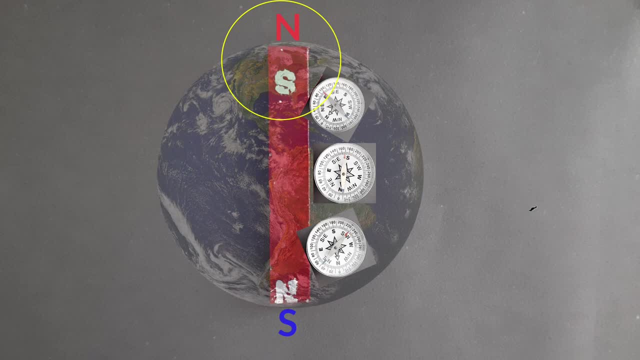 Ener繼續 lamps. i used warn of how nice this is for first talk. So does that mean that Earth also behaves like a magnet? Well turns out. yes, it does behave like a magnet. I know that sounds insane, but it's true. 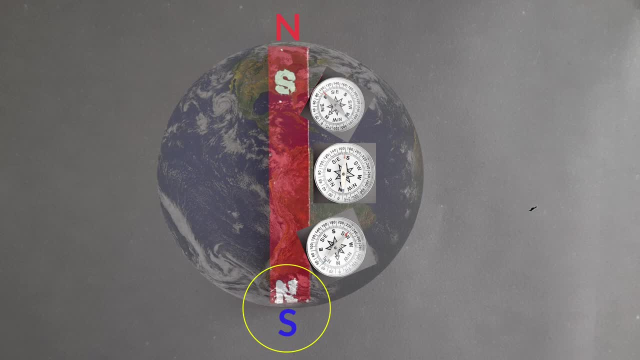 magnetic north pole of the earth. it lies near the geographic south pole of the earth. it can be a little confusing but you can understand it. by looking at how the needle of the magnetic compass moves in the top half in another hemisphere we can see the north pole directed towards a north 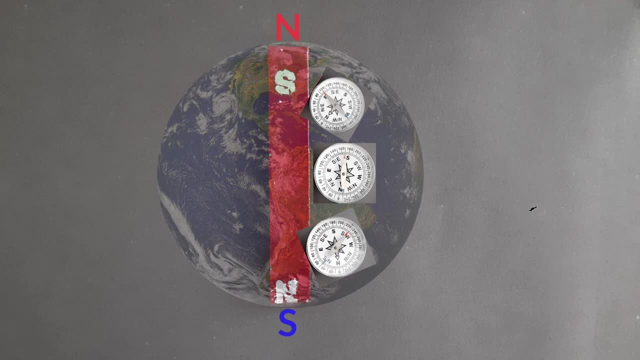 pole, the geographic north pole. but we know that the north pole of of a tiny magnet like a needle will always be attracted to the south pole of any other magnet. so the magnetic south pole should be near the north pole and similarly the magnetic north pole should be near the geographic south. 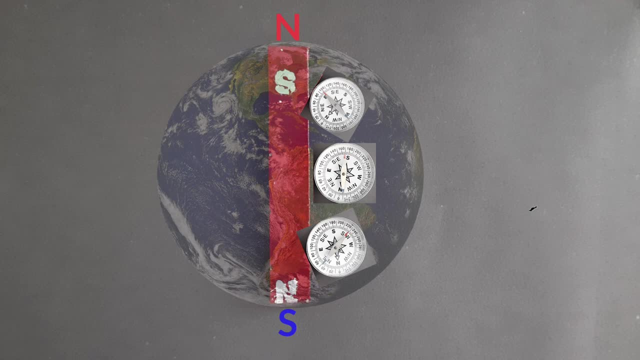 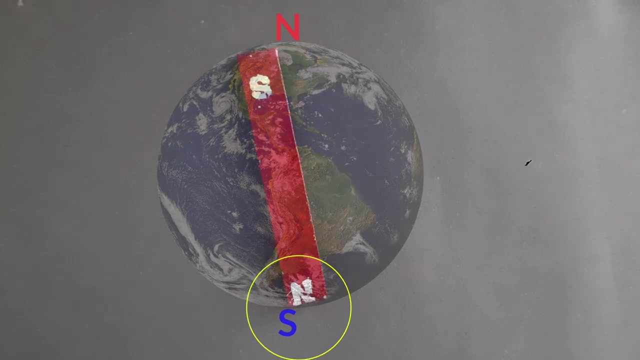 pole. now, because we're trying to visualize how earth behaves like a magnet, we can also be slightly more accurate and say that the magnetic south pole of the earth does not directly lie on top of the geographic north pole. in fact it is slightly shifted like this. so just by shifting, 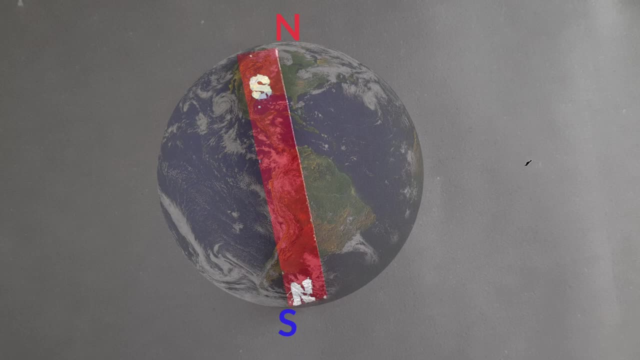 the magnetic north pole does not lie directly on the geographic south pole. you, lastly, don't think that there is an actual magnet inside the earth, right? the? the reason why earth behaves like a magnet, it's a completely, they're completely different reasons to it. it's, it's not. 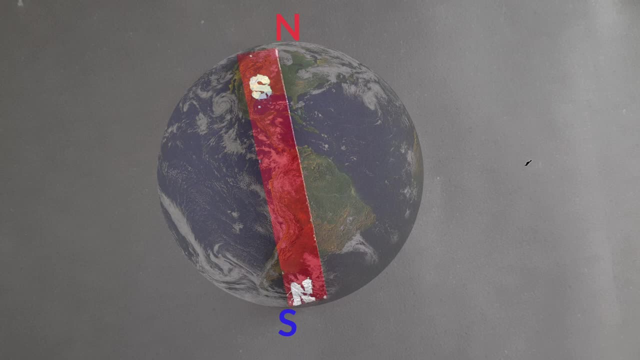 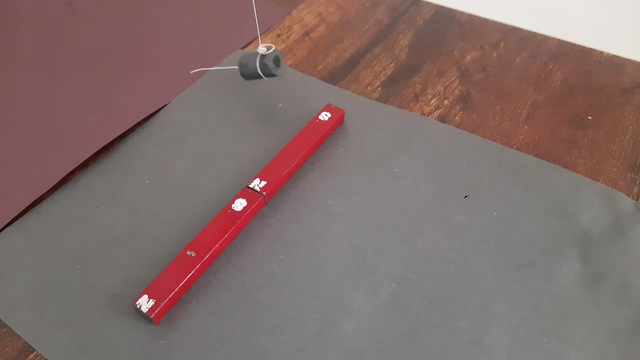 that there is a magnet, like a huge magnet, inside the earth. that's not the case. all right, let's, let's try and visualize this again now. let's take a small piece of magnet. so i want you to observe how the small black magnet moves as i move it along the length of this long. 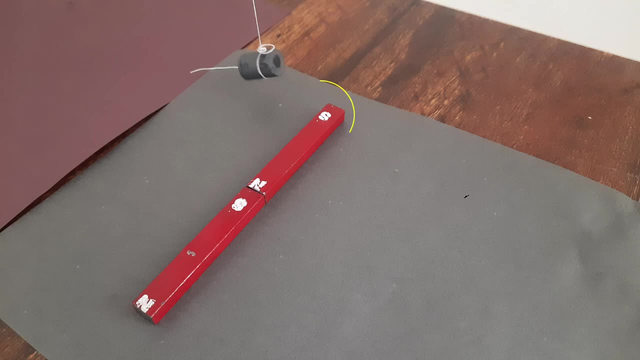 barbicane that i've created. so this, this end right here is a south pole, this end right here is a north pole, and in between you can imagine these two poles are cancelling each other. so this behaves like a long bar magnet. now notice, notice how the tiny black magnet moves. so right now, this end is being